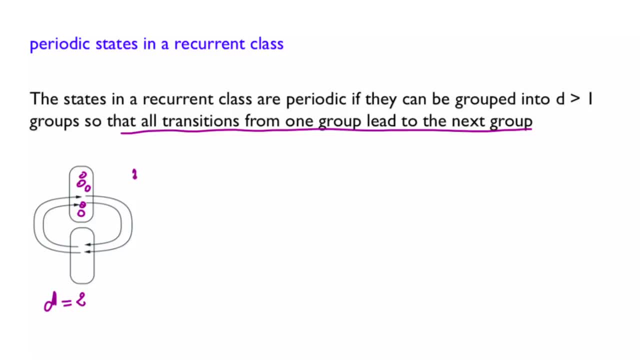 started in one of these states. here, at time n equals 0,, then at time n equals 1,, it would be here. And then at time n equals 2,, it would be here. Times n equals 3,, and so on and so forth. 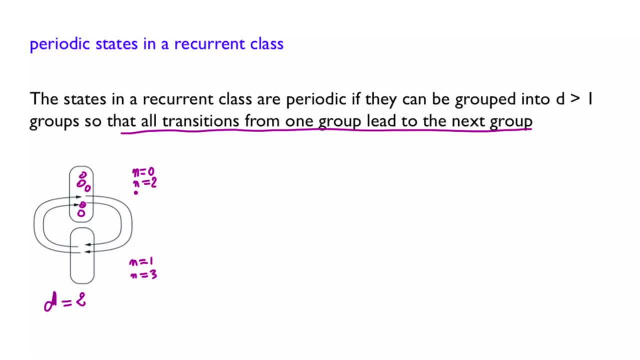 So every time you would have an even number. then you are guaranteed that the Markov chain will be in one of these states here. Clearly, with this kind of structure it is impossible to have convergence of the steady state probabilities. This is another example where you 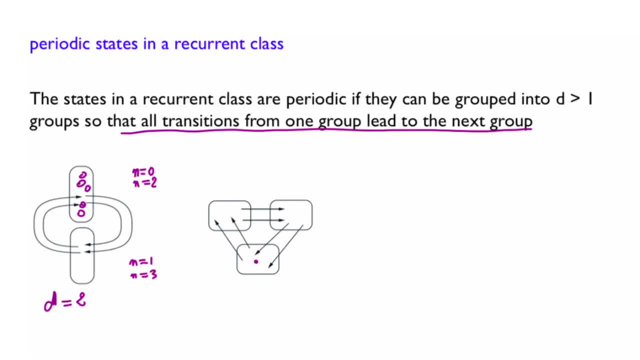 would have a structure of a diagram in which you have a picture, And then you would have a period of 3 here. So in that case, here d equals 3.. So here again, if you are in one of these states at a given time, then at the next time. 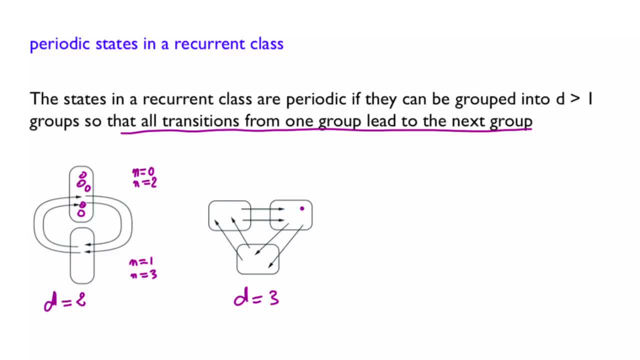 the following transition will guarantee to bring you in that group, And during the next transition you will go to that group And then again, here And again. you will have this kind of behavior in a very systematic way. So if you started here at time, n equals 0,. 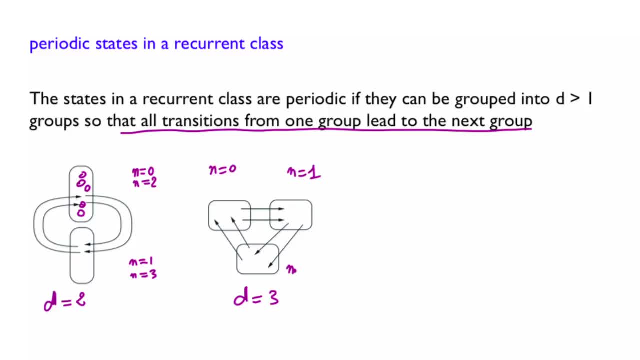 you would be in that group here. You would be here at times n equals 1.. And you would be here at n equals 2.. And again n equals 3 here, n equals 4.. n equals 5,, 6,, 7,, 8.. 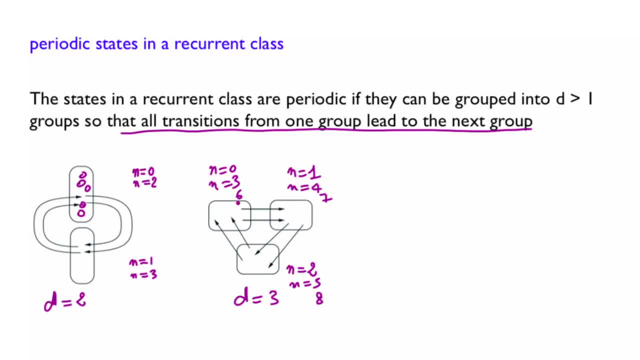 And you see the pattern If you look at any time in the future. if the time is of the form 3 times k, for any k greater than or equal to 0, you're guaranteed that your chain will be in one of these states. 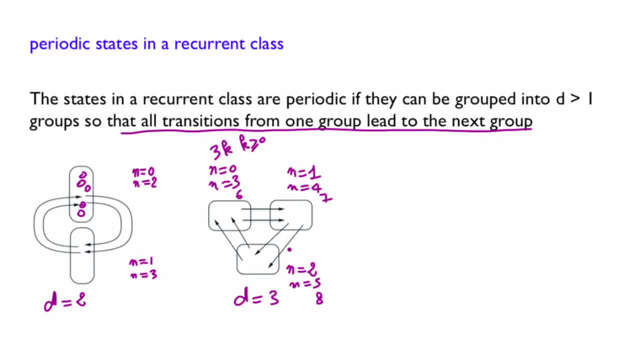 Otherwise it will be here or here. So here again, you do not have convergence of the steady states, Because if you are told that you start in one of these states here, then you know that whenever you have a time that is of the form 3k plus 1, you will be here. 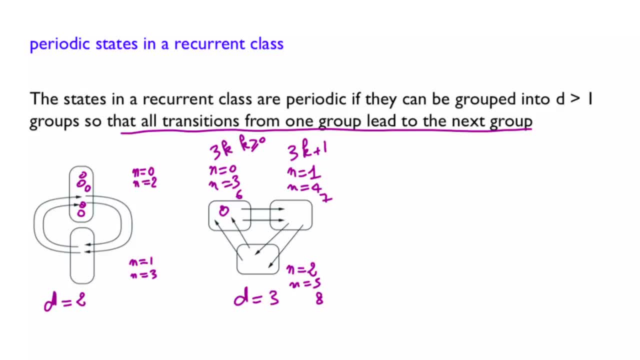 And so the probability of being here will be 0.. All right, So we have been able to explain a little bit what a periodic state is using this definition. Now, given a Markov chain, how can we tell whether a Markov chain is periodic or not? 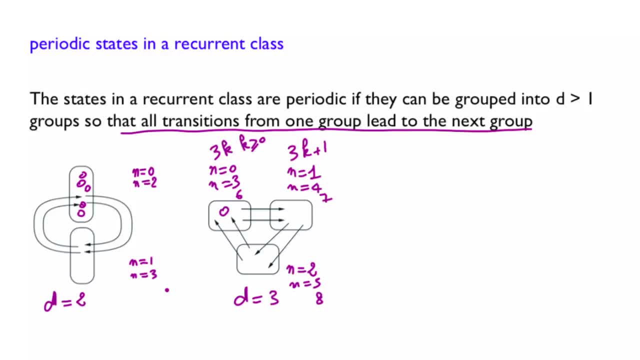 There are, in fact, systematic ways of doing it mathematically, But usually within the types of examples we see in this class. most of them, it will be easy to see. we just eyeball the chain and we tell whether it's periodic or not. 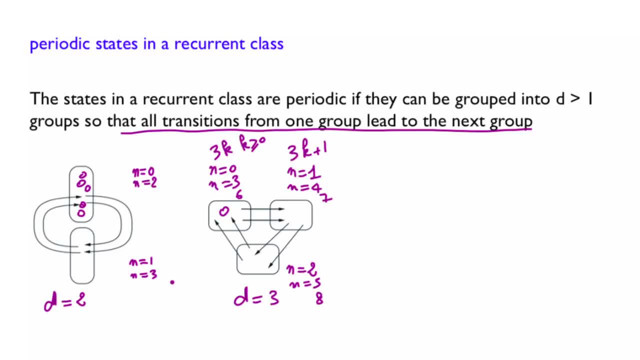 So let us see if it is that easy to do. and consider that chain here. OK, So let's see, Is this chain periodic or not? I will give you a couple of seconds to think about it. Now I'm going to help a little bit. 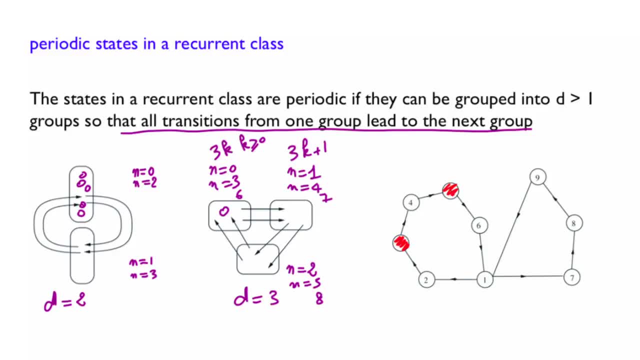 I'm going to just decide that this one will be red, this one will be red, this one will be red and this one will be red. Now I'm asking the same question: What do you think? Well, from the structure, it is clear that this Markov chain 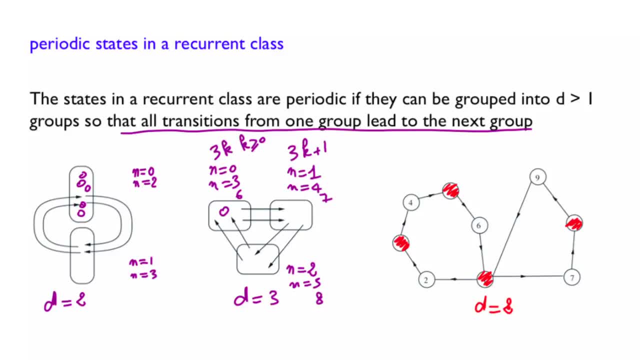 is periodic and has a period of t equals 2.. In some sense, the red state here could be one of this group. These are the red one. The white here would be those here, And it is clear if you look at this diagram. 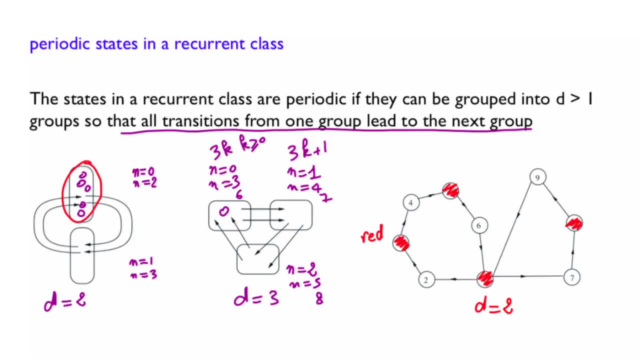 that whenever you are in a red state, at the next transition, you are guaranteed to be in a white state. From this one, you will be in white. From this one. you will be in white. From this one as well, and from this one as well. 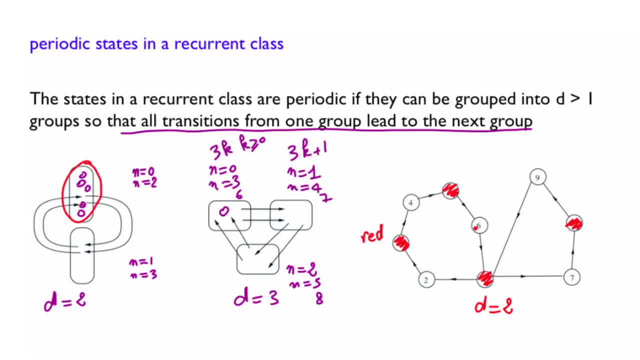 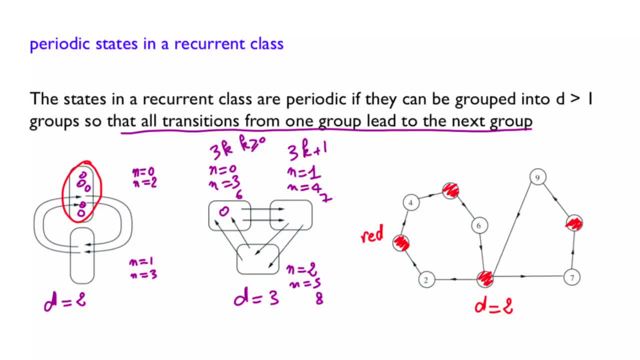 and decide if a Markov chain is periodic or not. If you have, for example, lots, of, lots of states, you might have some trouble doing this exercise. On the other hand, something very useful to know. Sometimes it's extremely easy to tell. 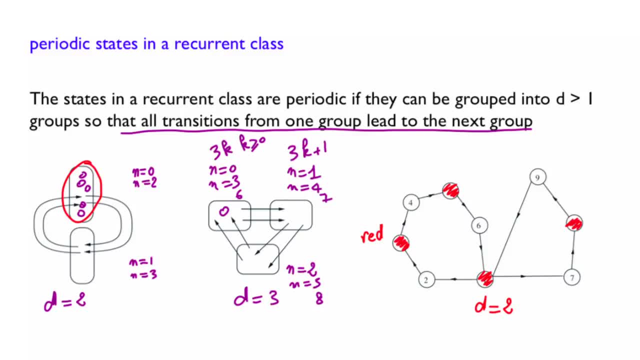 that the chain is not periodic, even if you have a lot of states. What is that case? Well, look at this case here and suppose for a moment that you have a self-transition here. Well, in that case you would have a transition.